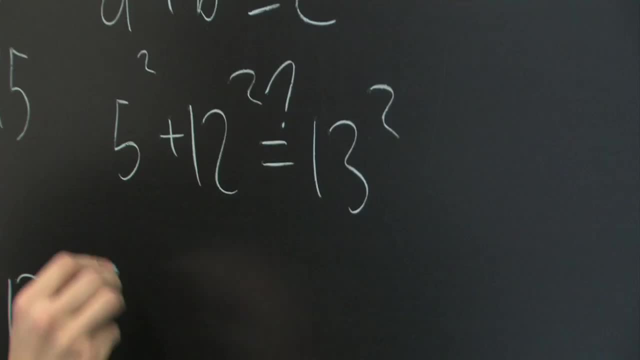 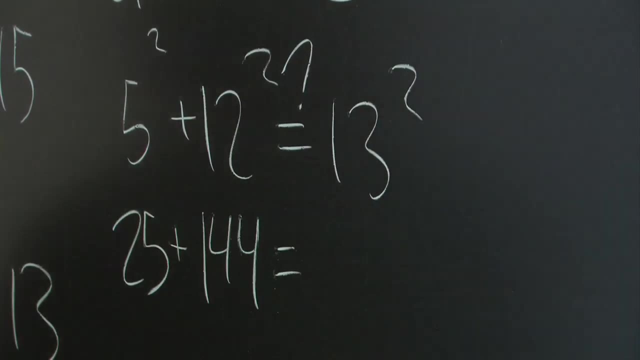 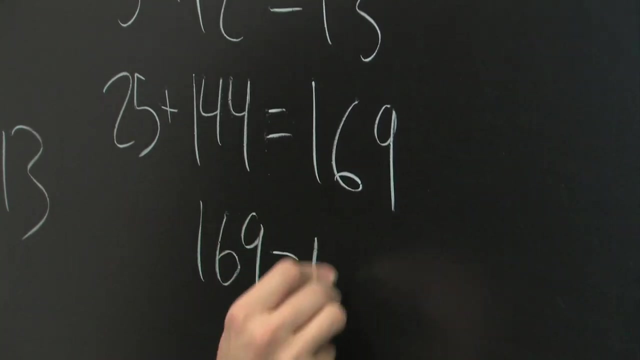 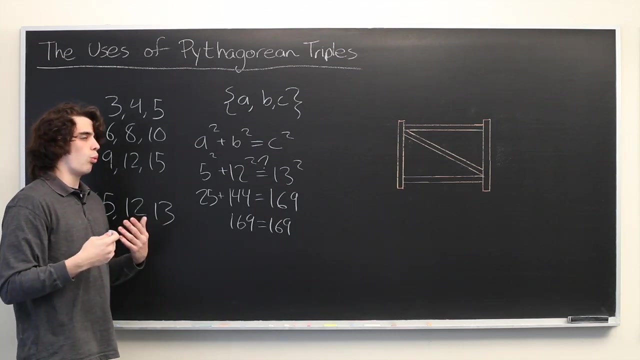 squared. If you're not sure, just do the computation. Five squared is twenty-five, twelve squared is one hundred forty-four and thirteen And thirteen squared is one hundred sixty-nine, And it is indeed true that one hundred sixty-nine is equal to itself. So that is a Pythagorean triple. But the question remains: what good? 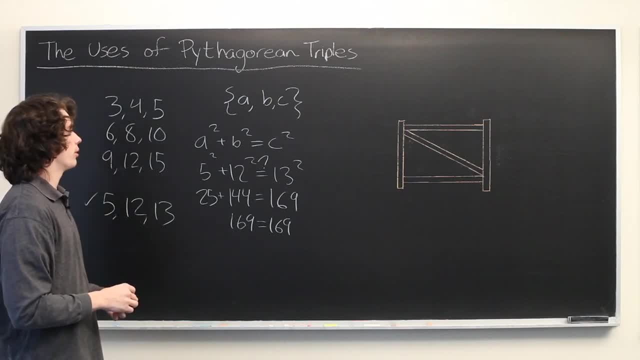 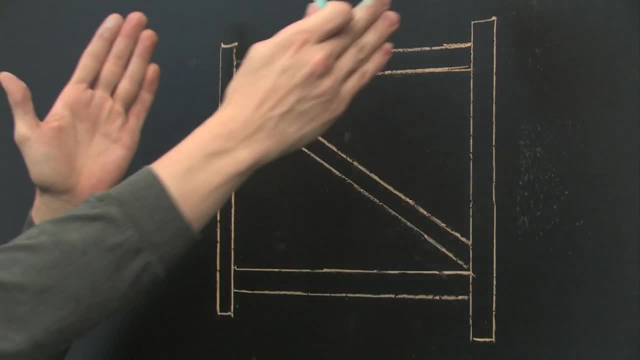 is it to know about any of these? When would it ever come up in the real world? And here's an example: Let's say you're building a fence, or designing a fence, where there are going to be posts, horizontal beams and then cross beams. 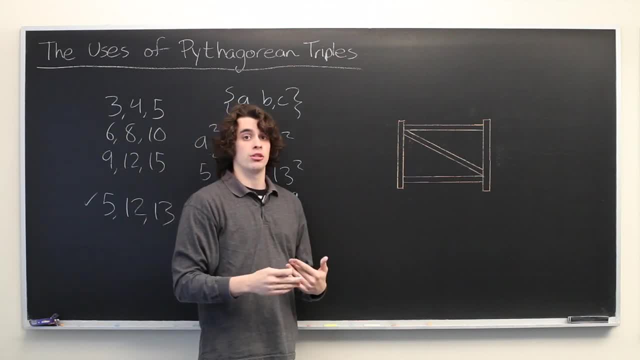 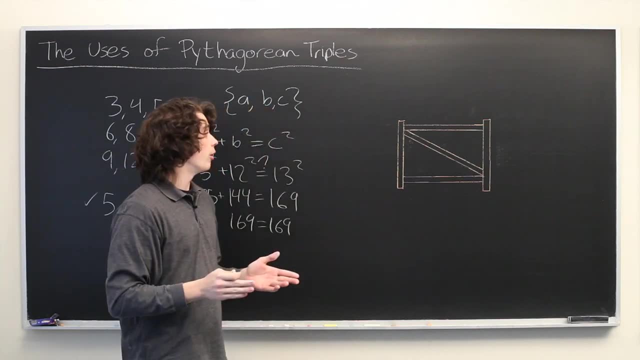 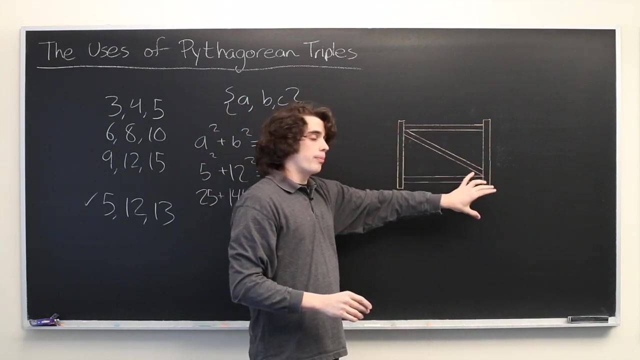 And let's say that the type of lumber that you're using to build this fence comes in units of maximum length of sixteen feet. And what you want to know is: can you design this fence in such a way that all three measurements will be integer: multiple of feet, but less? 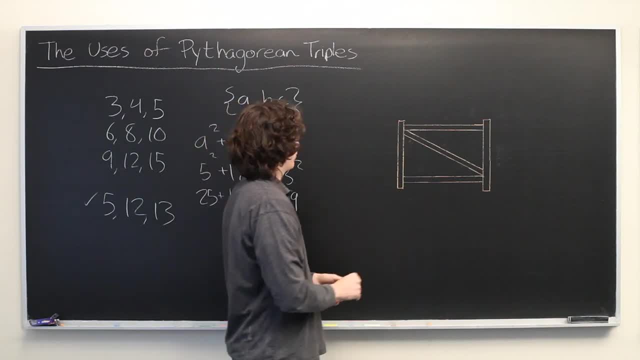 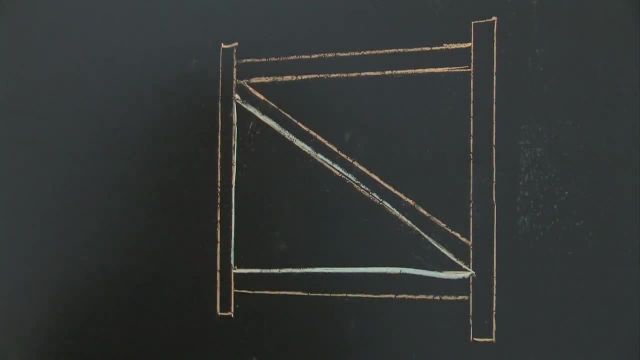 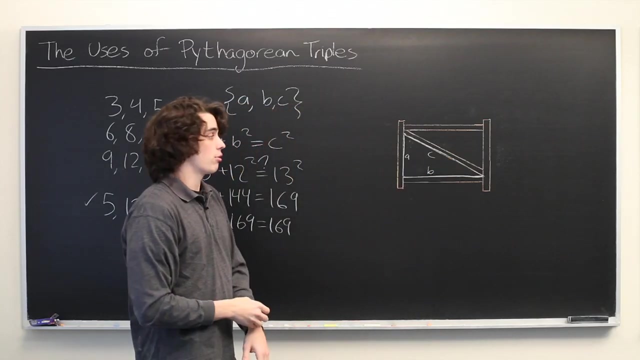 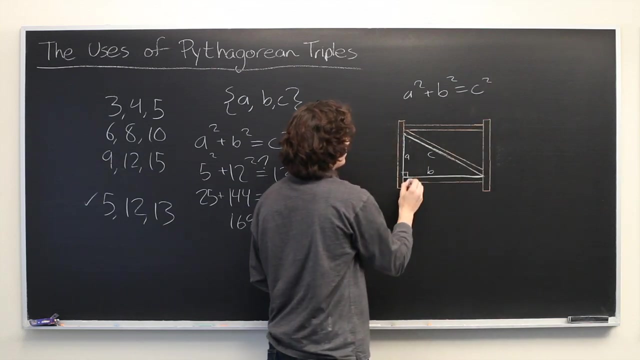 than sixteen feet. And well, the answer is yes, If you just imagine this as being a right triangle. And we label this a, b and c. Well, by the Pythagorean theorem, a squared plus b squared equals c squared in a right triangle. But that's exactly what we have here. So all we 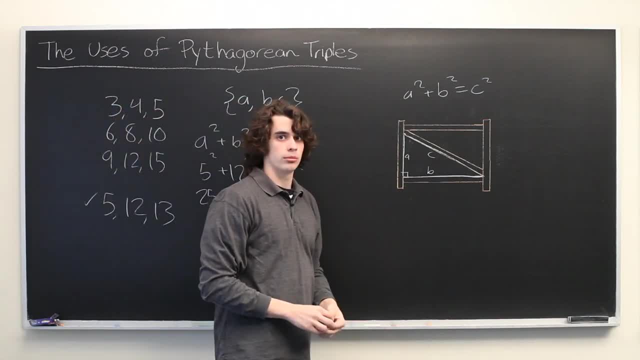 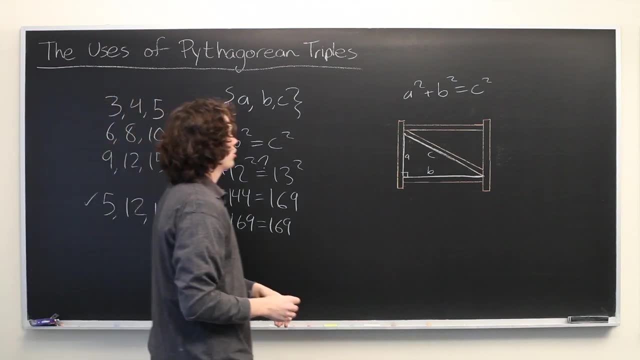 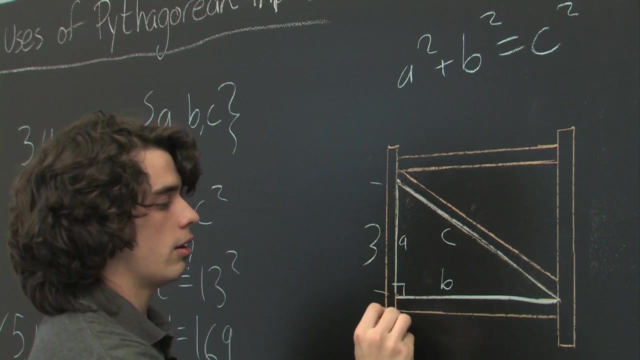 need is a Pythagorean triple to satisfy this equation, in which all of the numbers are less than sixteen. But we've got a handy list right here. So what this tells us is that we could do, for example, three, four and then a hypotenuse. 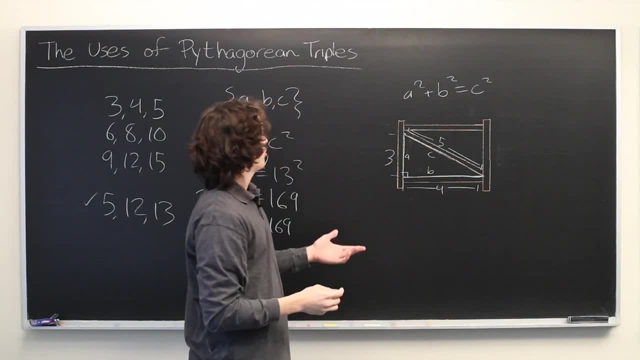 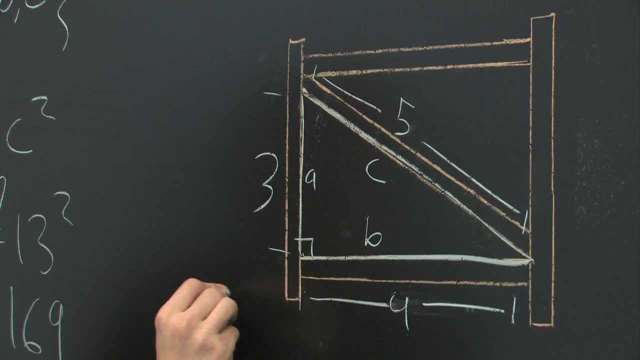 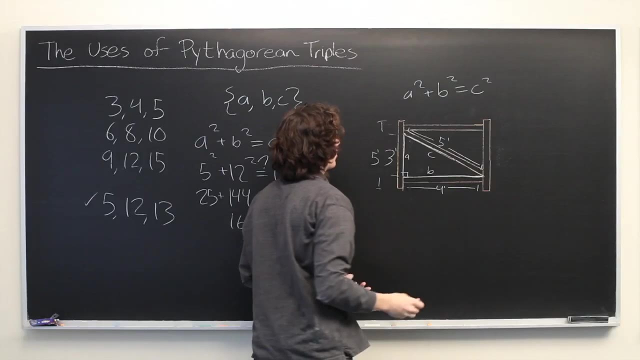 of five feet And if you want to be slightly more precise, since this isn't the entire length of this post, you might extend this upward a little bit and say that this entire thing is five feet, Or you could, if you want to make it a somewhat longer fence, you could use the five twelve.